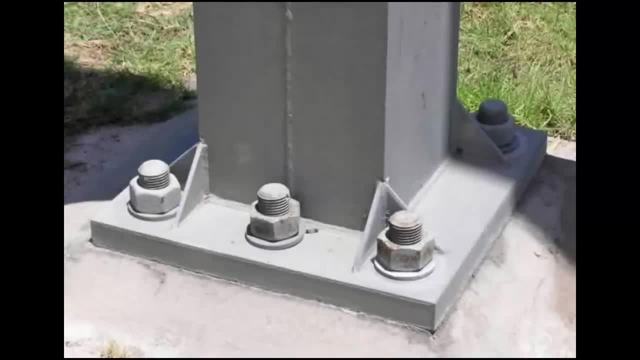 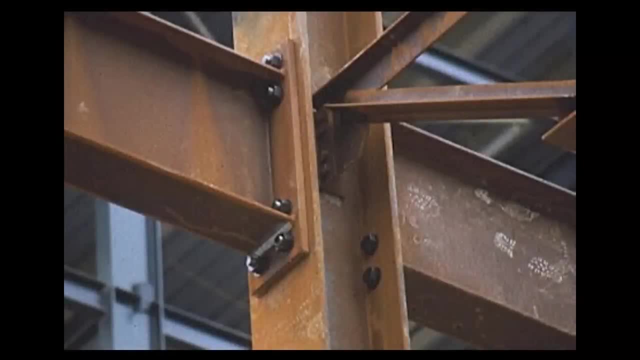 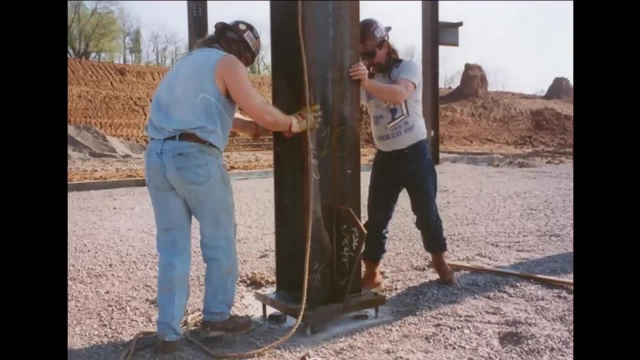 Now, regardless of the shape, each column will have a base plate in some form or fashion for attachment to the anchor bolts and connection points for the upper structural elements. During initial assembly, the columns are loosely attached on the anchor bolts to allow for easier assembly of the horizontal structural elements. 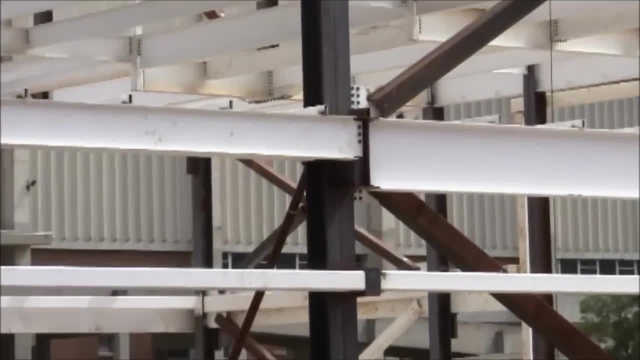 During initial assembly. the columns are loosely attached on the anchor bolts to allow for easier assembly of the horizontal structural elements. The horizontal structural pieces will consist mainly of I-beams. However, in certain areas tube steel will be used for the horizontal elements. 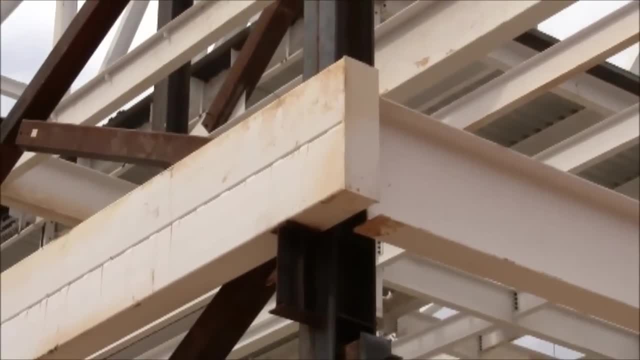 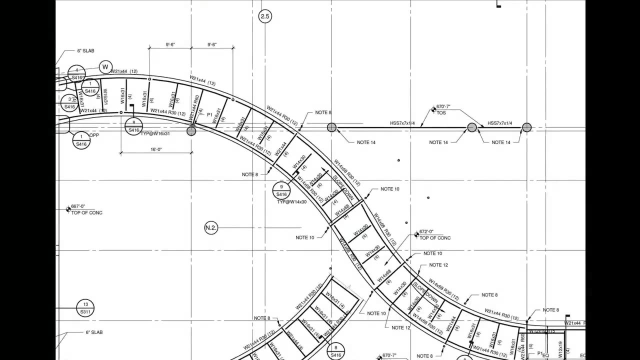 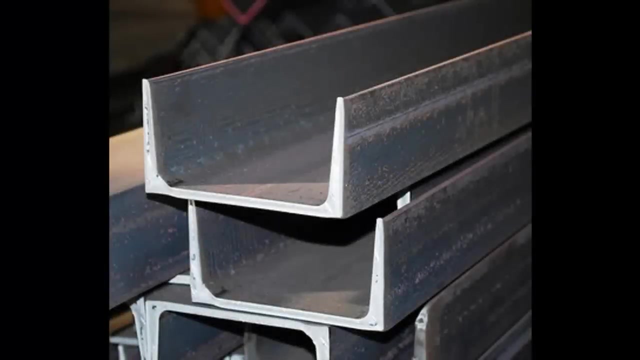 Tube steel is also commonly used for cross-sectional bracing within the framework. Just as with columns, the nomenclature for these pieces is typically the same In cases where the loads are not that extensive, such as canopies and beams over doorways. 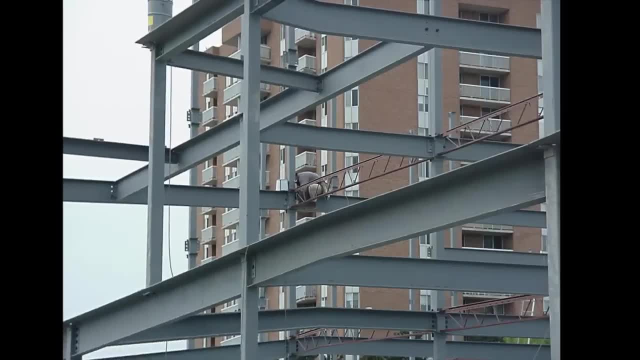 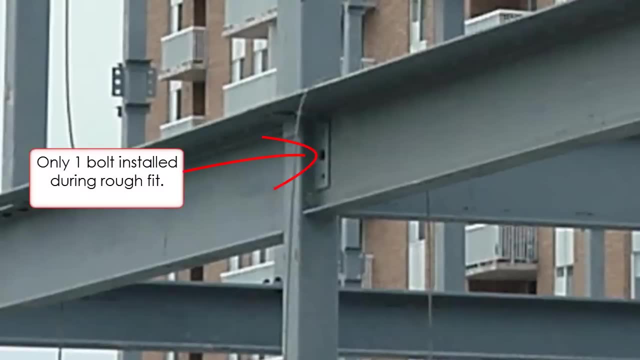 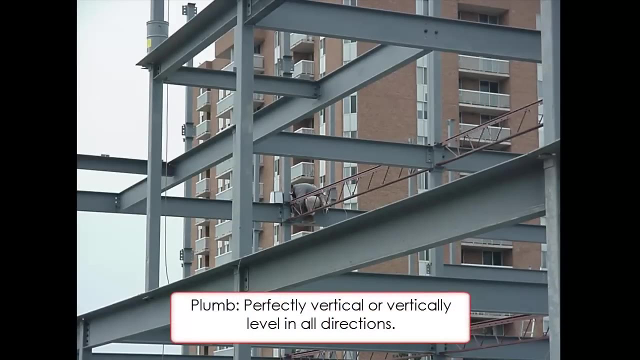 a steel channel may be used Again during installation. these pieces will all be loose-fit until the entire framework is together. Once assembled, the steel erector will go back and begin to plumb all the columns and square up the horizontal sections. 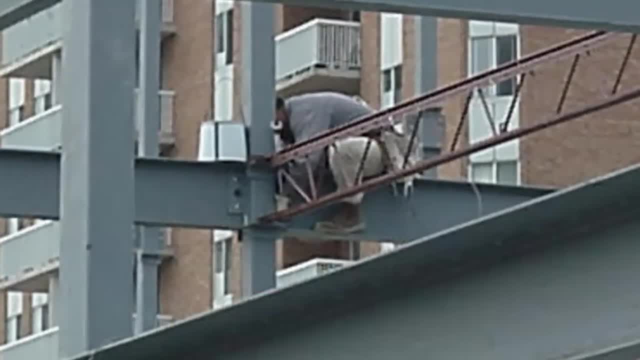 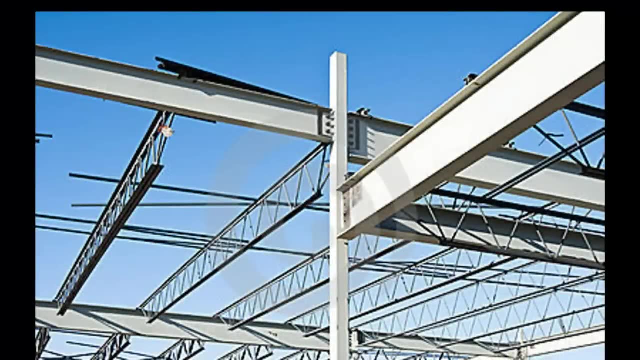 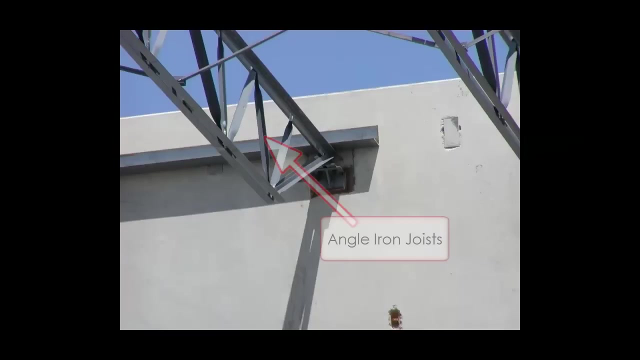 As this is done, they will tighten up the connections and install any bolts that were left out during the rough assembly phase. This makes the primary steel ready for assembly. In most cases, these are bar joists. Bar joists are fabricated in various shapes and sizes, which we will discuss in another video. 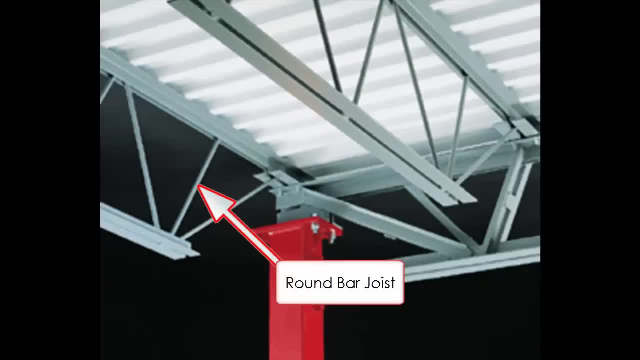 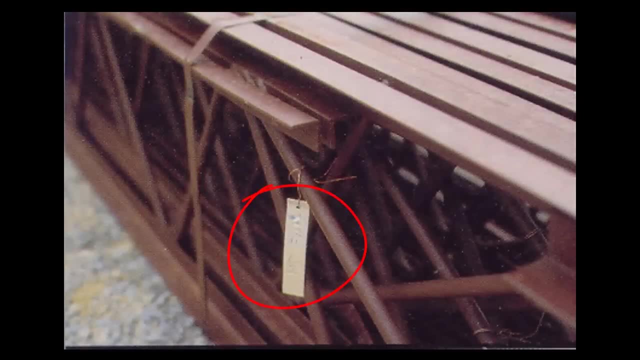 Each joist is typically tagged, identifying its manufacturer, sizing and area of placement within the project. As you can imagine, with most projects, there are a lot of different bar joists being used, So knowing where we want to place the joists and where we want to place them is important. 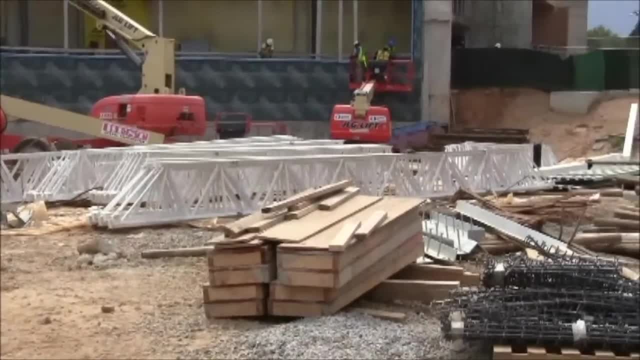 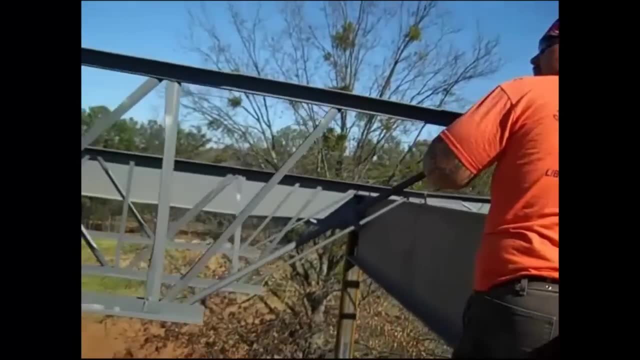 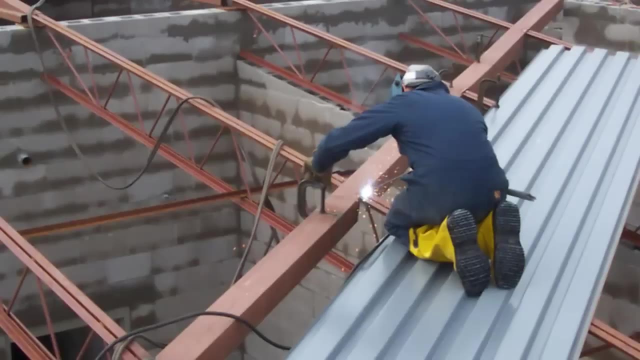 For example, in this project we are going to use a bar joist. Knowing where within the project those joists fit make it much easier for the ironworkers during installation. They can be installed using either a bolted or welded connection, or a combination of both.